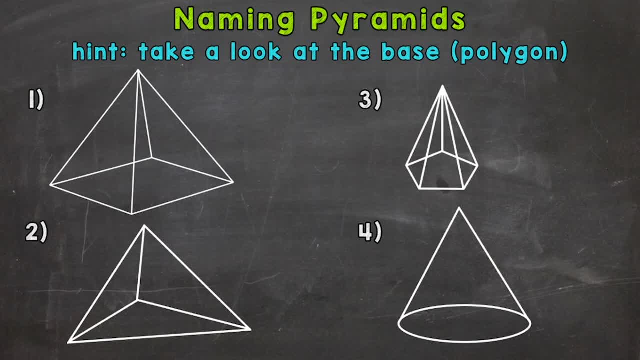 its specific name. A pyramid also has triangular faces or sides that meet at a point called the apex. So let's get into naming some pyramids. So we'll jump right into number one here. So the first thing we need to do is find the polygon face that that pyramid sits on, and that's going to be. 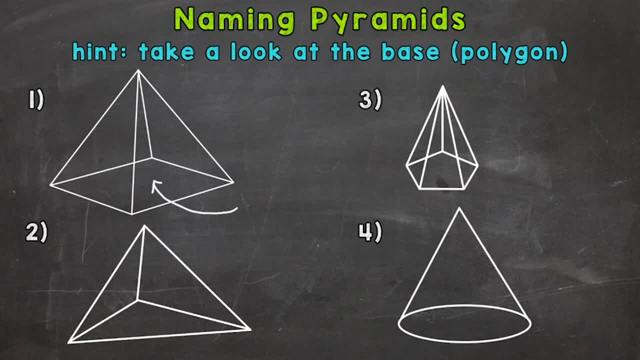 our base. So it's going to be the square down here, And I know none of the side lengths are marked, but they all are the same. So it is a square. So that's our base. And then we have the triangular sides or faces going around the pyramid, which meet at the apex. 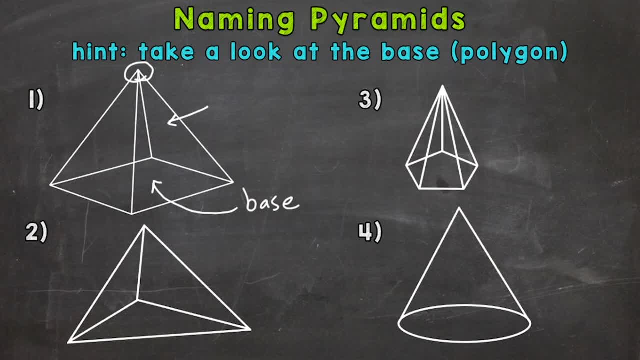 Okay, so we name a pyramid based on the base. So, whatever the base is, that's the specific pyramid And we have a square here. So for number one, we have a square pyramid. For number two- our base- we have a triangle. So, number two, we have a triangular. 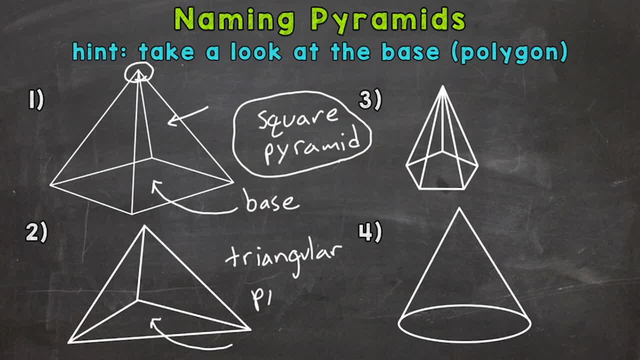 So this is a very typical pyramid, And I'll circle our name there. Number three looks like we have a pentagon base, So this is a pentagonal pyramid And, lastly, we actually have a counterexample that is not going to be a pyramid. 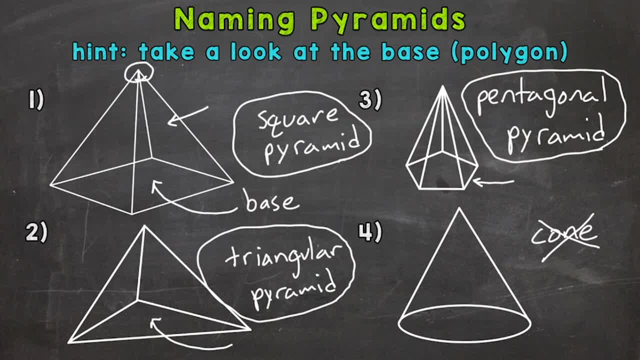 This is a cone, but it is not a pyramid. here's why Your base has to be a polygon. So we have an oval base here, which is not a polygon. A polygon has to be flat, which that oval is. It has to be closed, which that oval is But a polygon. 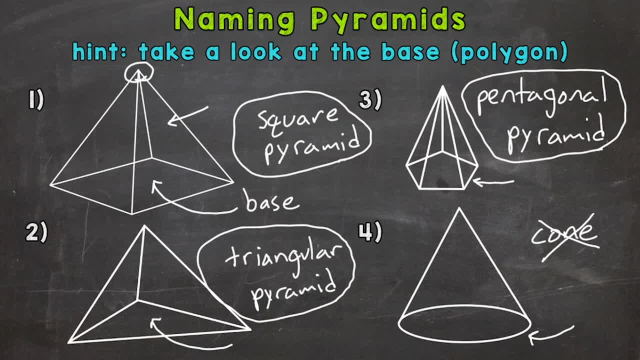 has to be made of line segments, so no curves, And that oval does not fit that description. So it's not a polygon and therefore not a pyramid. I do want to mention that these are not the only pyramids out there. The base can be any polygon And again we name a pyramid based on that polygon. 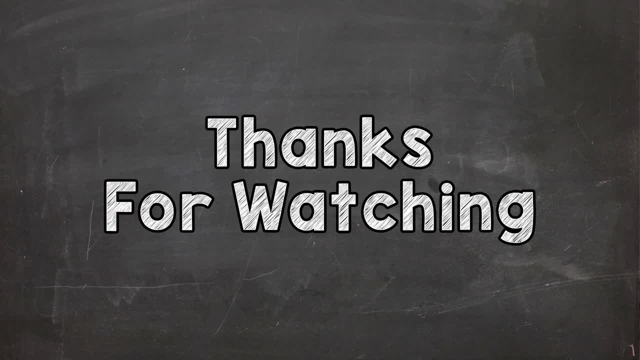 base. I hope that helped. Thanks so much for watching. Until next time, peace.